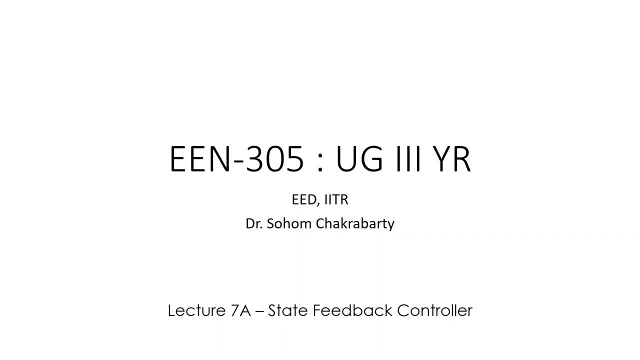 discovered about the system, all these ideas about the system we have come to know. Then we actually studied the system properties with respect to the control action also, And we try to understand the concepts of controllability, observability, reachability, etcetera And 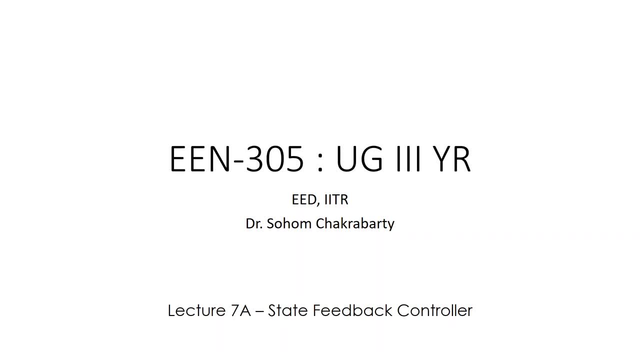 which deals with the system when we have the control action. there. controllability directly deals with the system when we are accessing the system, When the system is automatically running, so that the control projection of the system also has the manner which can also bePSR. so I have calculated the racing� variable. 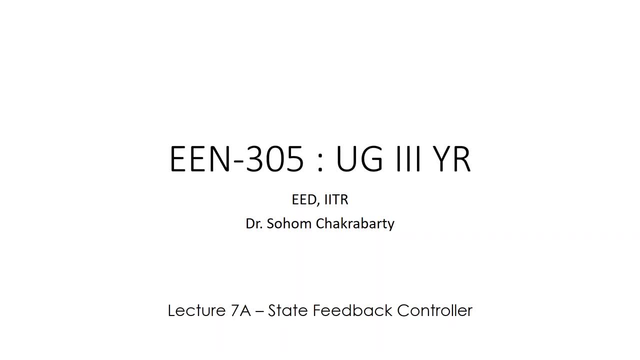 as actually the surface area. So this scheduler control action will act on the radiation, 可能 bePSR, but the resistance, this responsivity, have to take away from the source material. Thanks actually giving the control action there and we are trying to figure out whether we are. 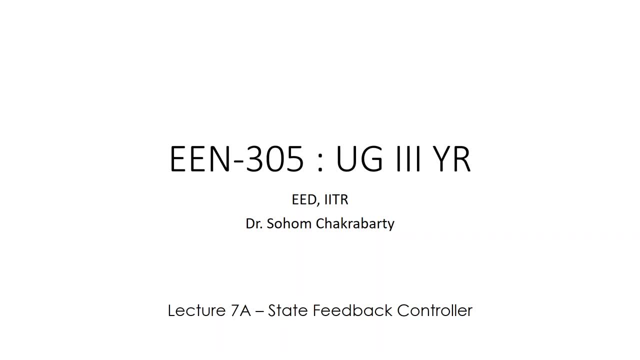 able to bring the system to a particular state, which is controllability, or bring or take the system to any any state in future, which is reachability. And also we we studied the conditions which would actually help us to understand the system, system like structural system, structural conditions- which is dependent very much on 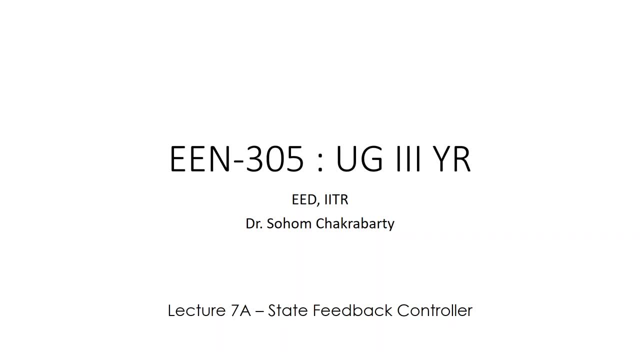 the A, B, C matrices, ah, So we those conditions about about the rank of the controllability matrix and observability matrix, we have, ah, we have studied, which actually actually gives us an idea about the controllability and observability Till now. actually, all these things has been studied. all these are basically we are studying. 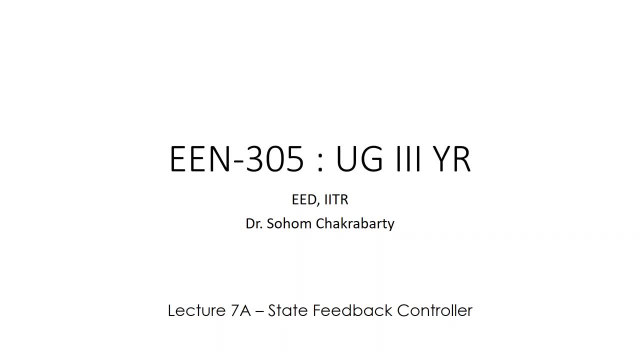 the. we are studying the system. So it is basically the analysis. we are analyzing the system, we are analyzing the, we are noting down its various features, etcetera, etcetera, but we are really not doing anything. ah, anything manipulative to the system, or ah, what should? 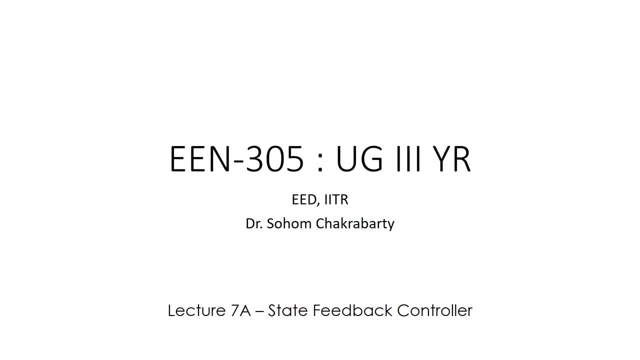 I say, I should say in this manner That we are, We are, we are not, not, ah, externally trying to influence the system. We are not trying to influence the system externally. We have understood what will happen if the system is is left in unforced condition. We have also understood what can happen if we actually 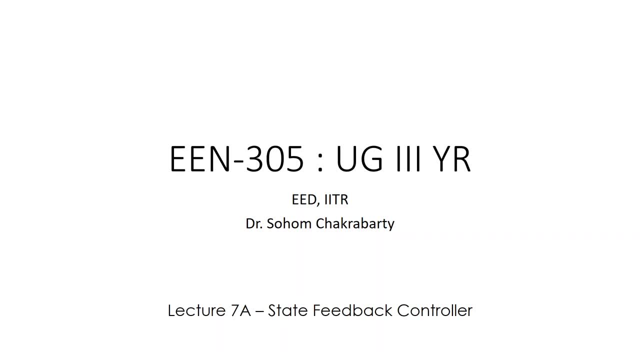 give a controller, ah, if we, if we actually give a control input, what can happen? whether the system is reachable or controllable, Whether we can observe the control of the system or observe that states by looking at the output. all these things we have analyzed all these. 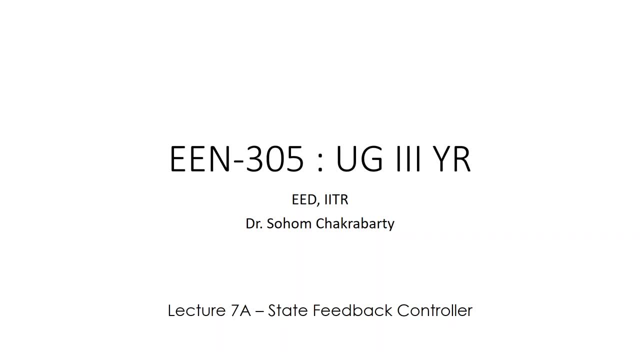 things come out from the structure, the state space, depreciation of the system. However, till now, we have not actually gone ahead and tried to manipulate the behaviour of the system, and that is what we are going to take up: this particular ah, this particular lecture. 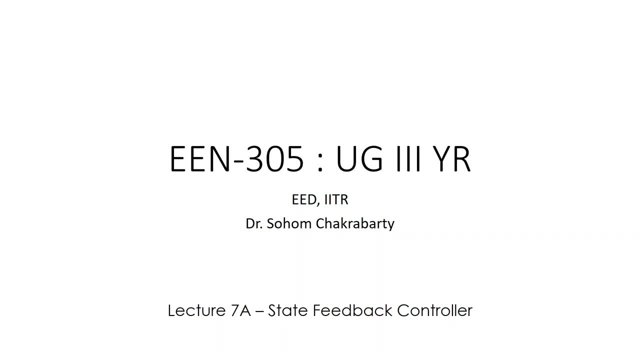 go and manipulate the behavior of the system, and when such a question of manipulation comes in, we are basically talking about supplying an external control in the system so that get some desired behavior from the system. the idea of a desired behavior is very important. you cannot just keep on giving any input, so you need to have some intention in mind. 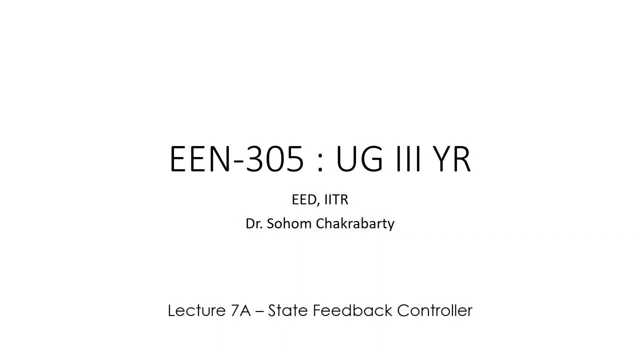 what you are trying to achieve. you are giving this input. so with that intention, if a proper, properly designed control input is given, then your intention will be achieved and whatever you want to want the system to behave as, whatever output you want or whatever performance you want from the system, 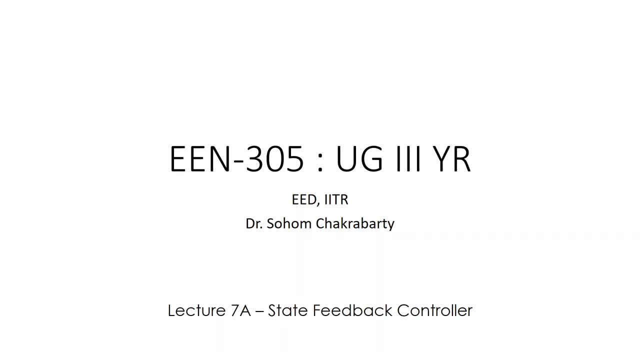 the system that you will get from. that is the basic aim of the control engineer, that is the aim of the control, although all the analysis that we have done so far is very important, otherwise this aim cannot be actually fulfilled. we have to do this- those analysis. but after doing this analysis, when we understand the system properties, we can now go ahead. 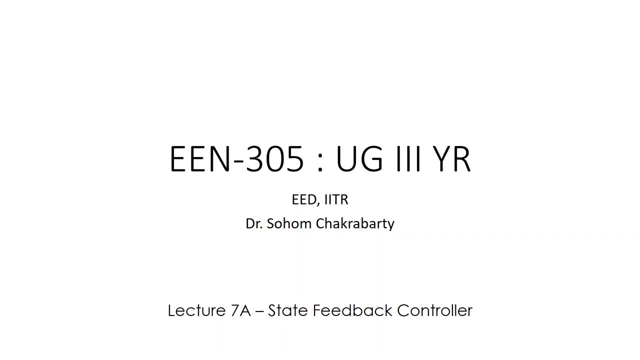 a step further and design the control input order to manipulate the system in a certain way So that it behaves the desired manner, it performs in the desired manner. So first we need to understand what are those desired behaviors which we are looking for. 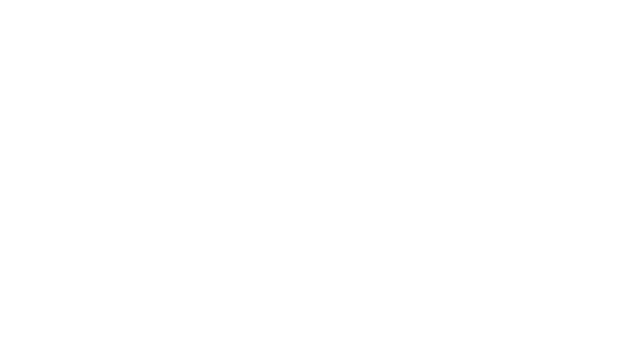 So let us Look at these problems. these are called the control problems and there are three control problems which you will see in any system. we are trying to actually target these three control problems. So control problem, these are control problem. either you are trying to stabilize the system, or you are trying to regulate the system, or 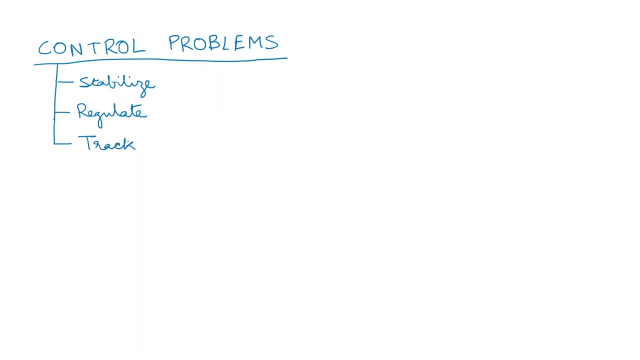 you are trying to track some or you make the system track something. These are the three control problems the control engineer is interested in, And these three control problems are distinct from each other. they are different from each other, so we need to understand what exactly these are In order to understand what exactly we need to do and when we understand. 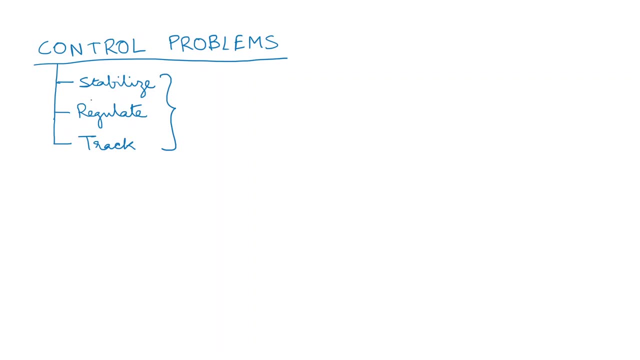 these three problems. we would actually discover that, though these three problems may not equal the problems, These may not equal the problems at a set level with the Mario Schroeder model, But when the plot sample is useful at those results of salvage into all Russian. 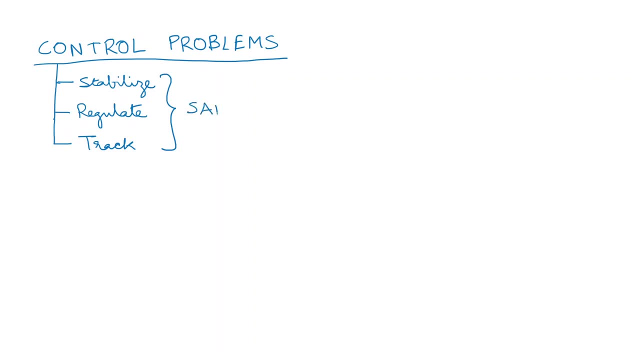 problems are different. they are actually the same problem. So we would actually try to solve these same problem. actually, what is the underlying commonality between these three problems? we will try to solve that, and that would make all these three problems get solved at the same time. So any problem you would give, you can solve it using the same method. 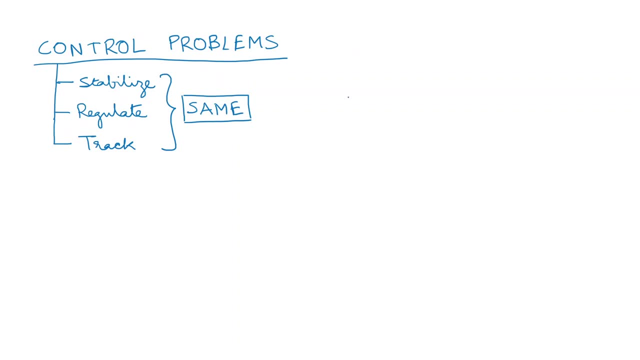 Let us understand what we mean by stabilization of a system. So in stabilization, so let us assume a state space. So for our purpose we assume a second order state space, but it can be any nth order. So there is a lag in writing. So anyway, this is the state space. 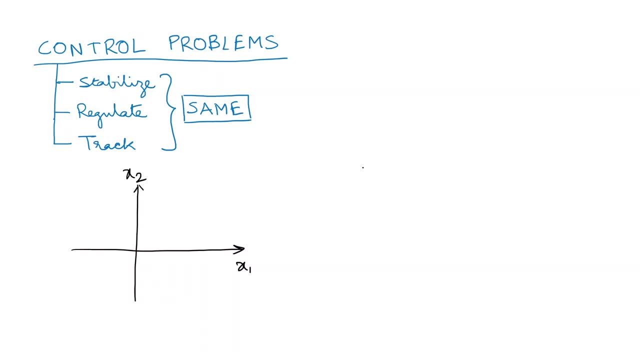 and if you think about the states, evaluation, evolution with time, So we have a a time graph and a states and a like and a trajectory graph. So this, whatever is in this particular graph will be the trajectory, whatever is in this particular graph is the trajectory. So this: 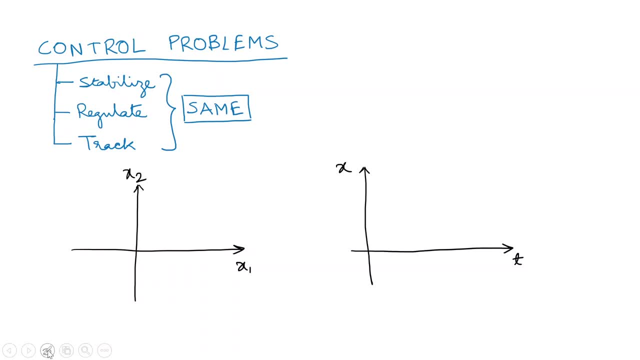 is the trajectory of the state evolution with time. So basically here we are talking about two states, but we can have any number of states. So what is the stabilization problem? The stabilization problem is basically the problem to come to the equilibrium point. that is stabilization Stable- the system is stable. that means the 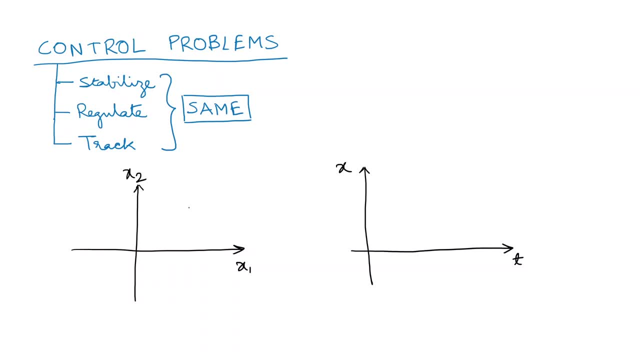 system is no more moving, the system is at rest. then the system is termed as stable. That means no matter where you are starting, you must come to the origin. You may come at with any trajectory. this is not so important in the problem of stabilization. So you can. 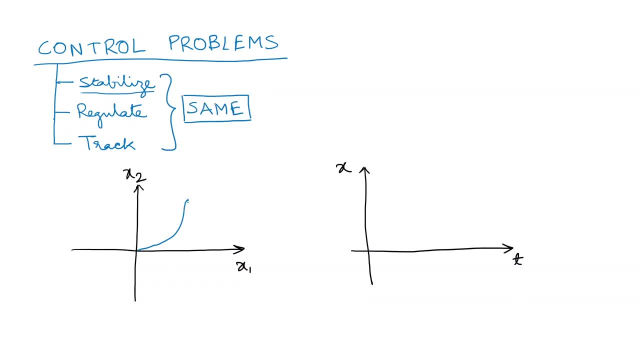 start from here. Suppose this is my initial point- you can come in this way, you can come in this way, So all these are valid. can come in this way, So 1,, 2,, 3, any trajectory you can take it. 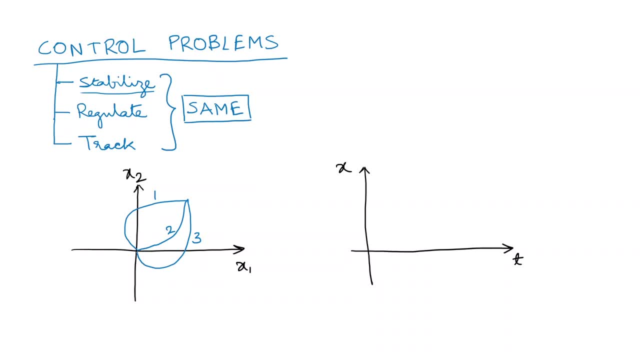 does not matter to us, as long as we are ultimately coming to the origin and then staying there for all future times. that is the stabilization problem. Stabilization problem means that your x- t tends to 0 as t tends to infinity. This is, as a particular name, called asymptotic. 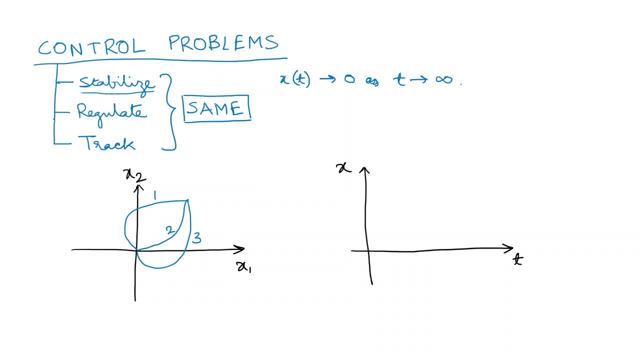 stability. at least we are trying to have asymptotic stability, the stabilization In this particular graph. what you will see? You will see that your states are in the order of x. I am drawing only one state, So there are two states, but drawing only one, it will. 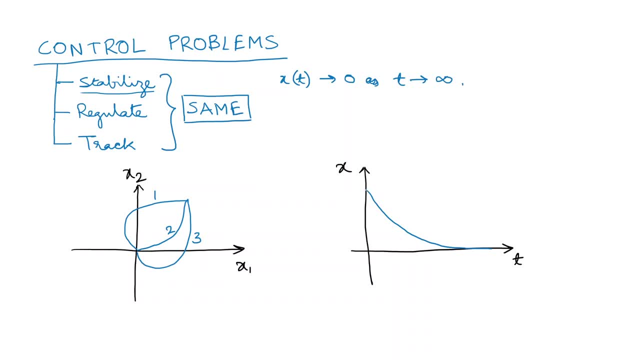 have a evolution like this. It can also have a like this. it can have a evolution like this. So any of this, suppose 1, 2, okay, so this is the problem of stabilization. So this is the problem of stabilization. 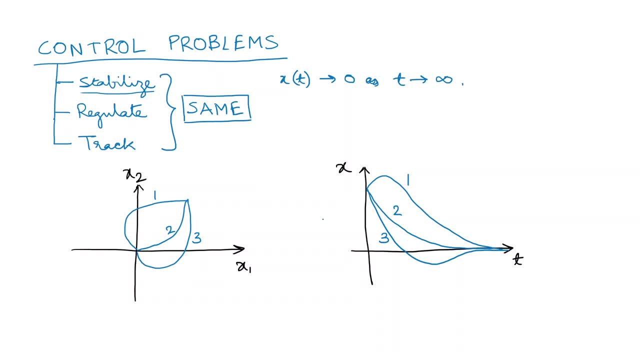 So this is the problem of stabilizing. Now, what is the problem of regulation In regulation problem? we are actually having some point where we want to go. This is the x- t desired position in the state space. You can start from the 0 position. you can start from any. 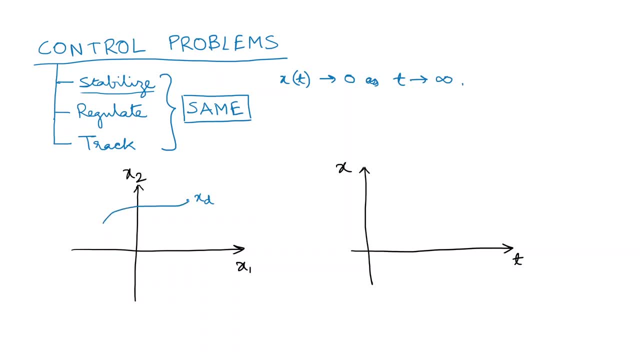 position. basically, Start from any position. you are trying to go to this position. This is your x initial, i, x, i to x d. you want to go How. you are going Through this route. you can go through any route, As long as you ultimately go to t and then remain there fixed. 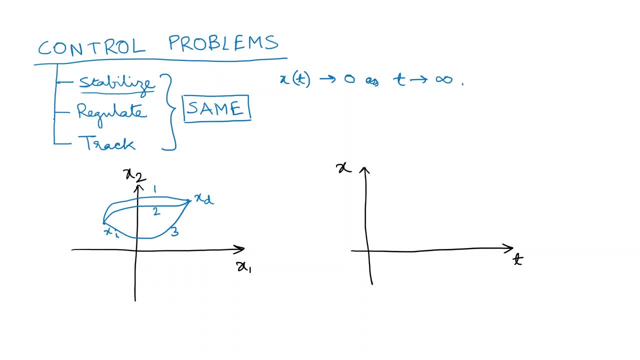 then it is fine with you. then it is fine with you. So here you will have a x d point and I can start from anywhere. I can also start from 0.. So let us start from some point other than 0 here. So I can come here like this: I can come here like this, I can come. 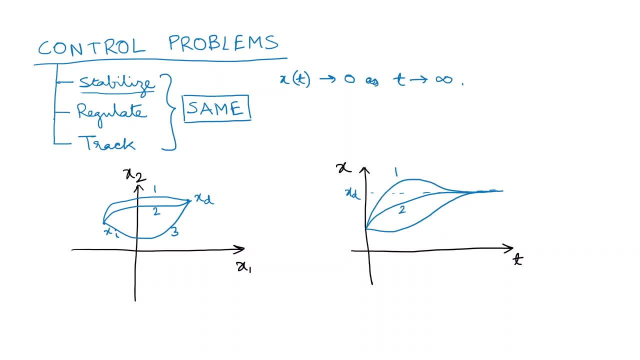 here like this: all these are values. This is the problem of regulation Here x t tends to x d as d tends to. What is the problem of tracking Centripetal? So what is this? First of all, we can say that x? t 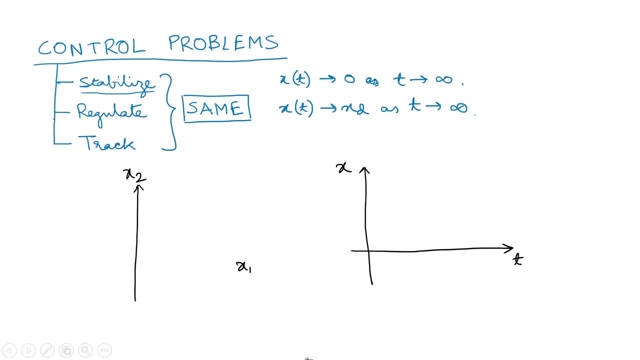 tends to x, d. What is the problem of tracking? Centripetal, Centripetal, centripetal, So remove the axis here. The problem of tracking? the problem of tracking. there is actually a desired trajectory in this case. So first stabilization. there a particular place has. 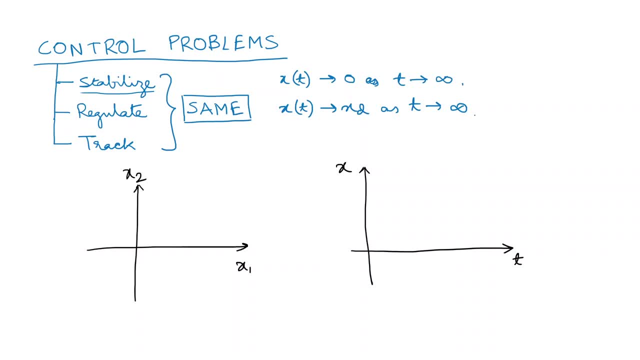 to be reached, which is the equilibrium point. the equilibrium point has to be reached in stabilization, In regulation. any point can be reached, but even other than the equilibrium point, but that point must be constant, So you have a particular destination to each. 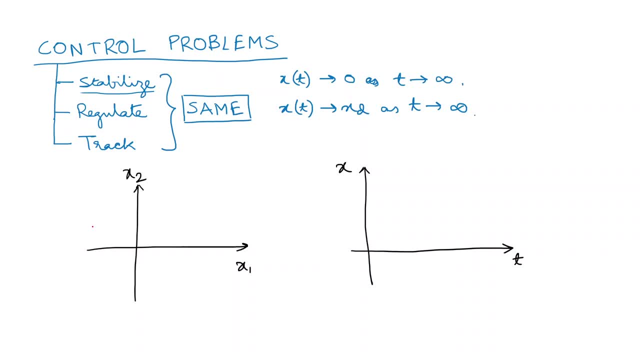 Now what you are doing. You are trying to take a trajectory here. So suppose I have some initial value- let us assume this 0 for this, for example. suppose I want to take a trajectory here. So I am taking the Hamilton's approach and I can cover my, my, my state space. 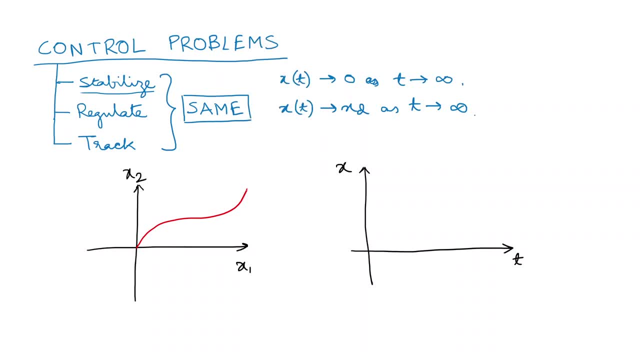 like this, and this is the final. this is the final position. I want to go in this route. I want to take. So my X1: you see X1 is taking so many, so many values with time. X2 is also taking so many, so many values with time. So X1 is going in this direction and X3 is. 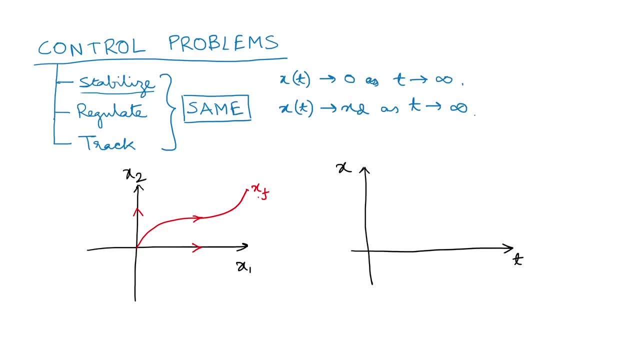 going, and so X3 as well. So, whether so many, so many values at the same time, or I can, x 2 is going in this direction. So it so when you actually actually draw it. so this is exactly the trajectory that I wish to take. basically, this is exactly the trajectory. 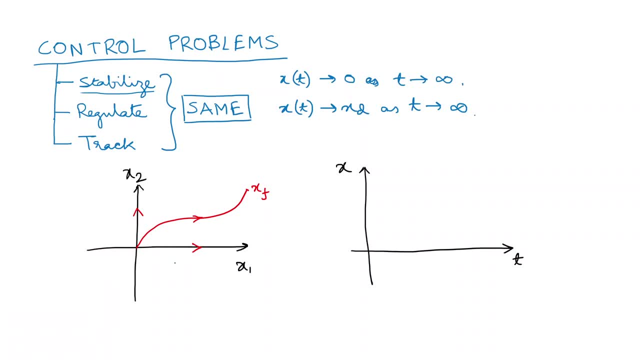 I wish to take. However, I may have started from somewhere other than the origin. also, suppose I start from this point, then what is my desired is that I track the trajectory as soon as possible and go like this, So you can have some controller which follows. 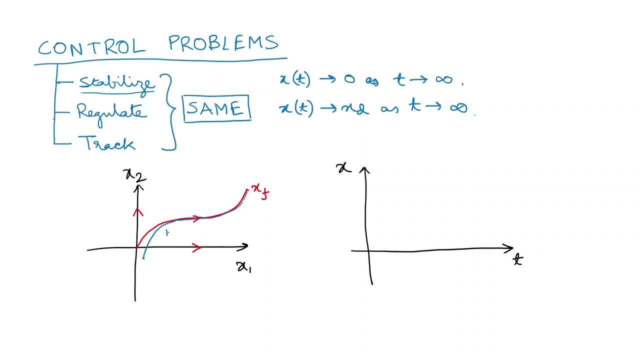 this particular blue trajectory which I indicate with 1, you can have another controller which will follow, like this number 2.. So all these different actual trajectories will depend on the actual controller you are using. the desired trajectory is the red one. ok, Now. 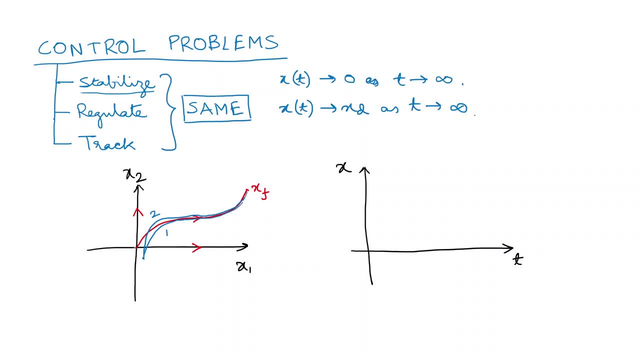 it may so happen that if you start from the 0, which is the starting point, even then you might not follow this trajectory exactly, So you might be deviating a bit and then start to follow. might so happen. all depends on your controller. ok, In this graph, what you will have for a particular state, you will. 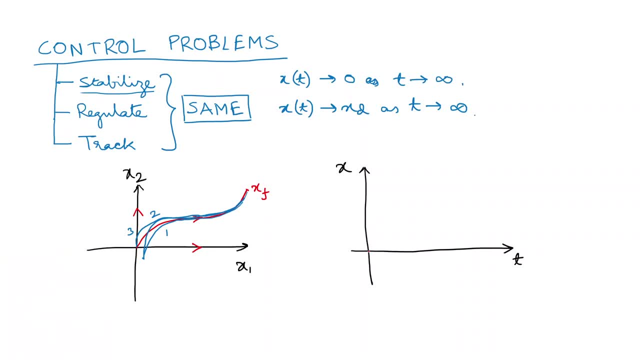 have a desired evolution. you will have a desired evolution, suppose this is the desired evolution. you will have a desired evolution for x1, suppose for the, for the x1. I am trying to draw xf1, suppose. So this is my desired evolution, but what I may see, that some control input. 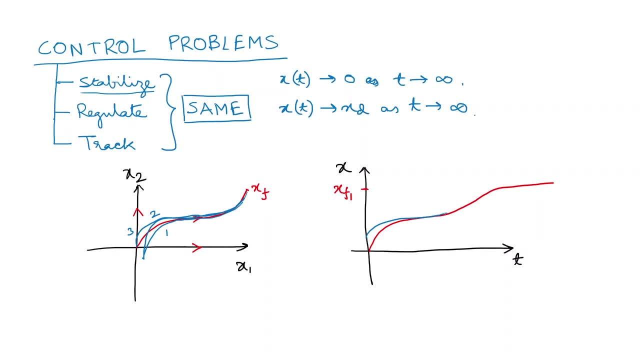 will make it like this and then it will track. some control input can make it like this and then it will track. And if the third one, which I started from origin it may also have some, also have some deviation, then it can be a track. But here the idea is tracking that. 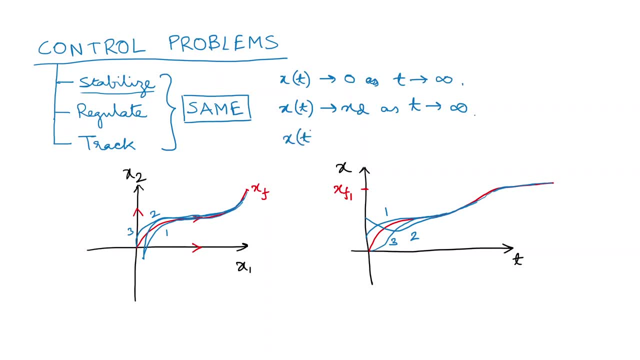 means x, t must end to some x, b, t. So it is not a constant anymore, it is a desired trajectory. So you know all the points in time of this trajectory. You know the time also. you know at you should reach this particular point at this particular time. that also you know. 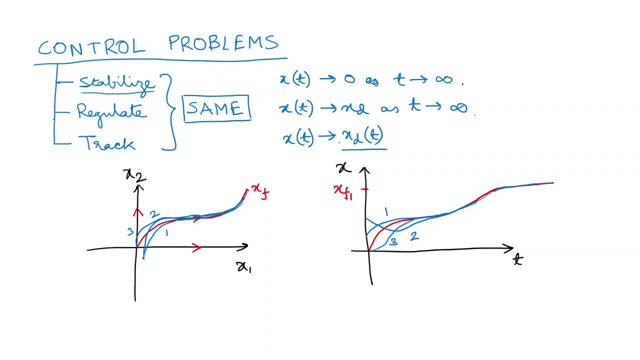 the entire trajectory is known And that you will want to actually follow your actual. this is your actual. you are trying to follow this and you want to do that as quickly as possible. but we write it like as t tends to infinity. That means with time I will reach the trajectory and then I will. 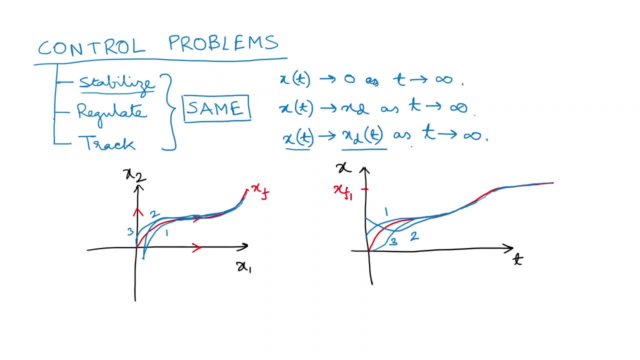 stick to it. ok, Obviously you can understand. as fast as we can reach, the better for us. but the definition wise we can. we actually define asymptotic convergence? All these are definitions of asymptotic convergence. The first one is asymptotic convergence to 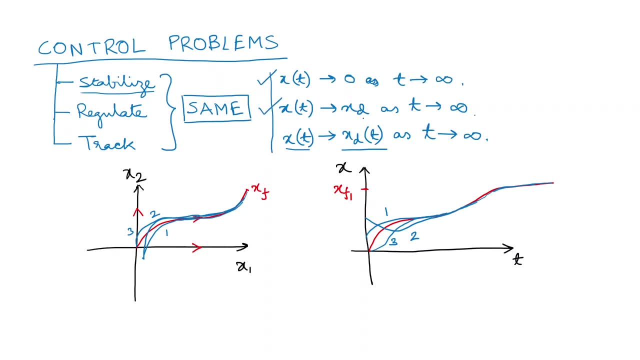 0,. second one is asymptotic convergence to a particular destination point. third one is asymptotic convergence to a particular trajectory. All these are asymptotic convergence to a particular destination point. So what is common to all these thing is the asymptotic. 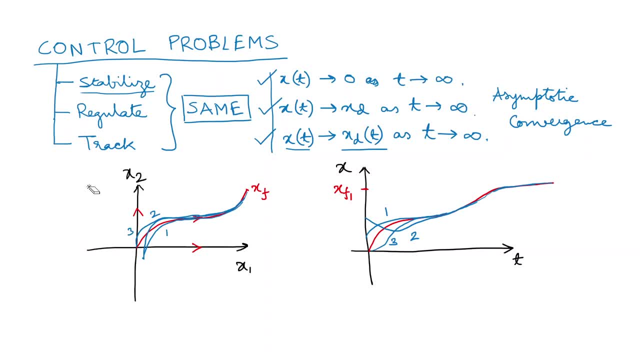 convergence, basically common to all these stabilization, regulation, etcetera, tracking. The common thing behind asymptotic convergence is the asymptotic convergence. If you think asymptotic convergence is not a calculus, This is actually possible If you have an asymptotic 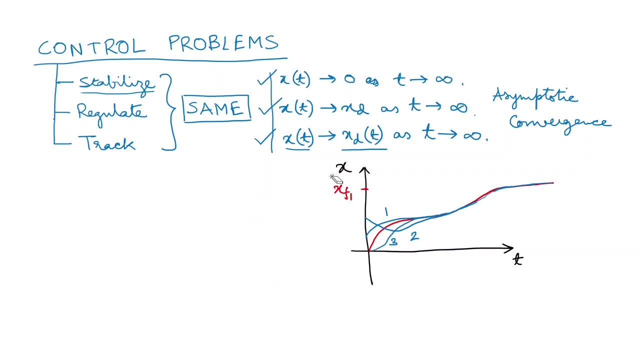 convergence behind all this thing is the asymptotic convergent, And you can, basically you have a state space representation like this. then in the first problem, you are trying to make x tend to 0.. 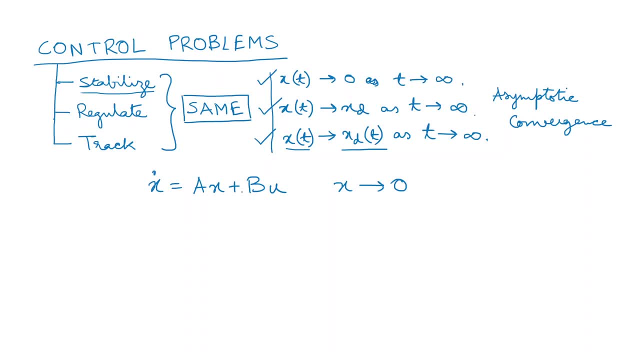 If you have a regulation problem, this is stabilization. if you have a regulation problem, then you are basically. you can basically construct a new variable, new error variable E as x minus x d, and then your intention will be to make error go to 0, right, Your intention. 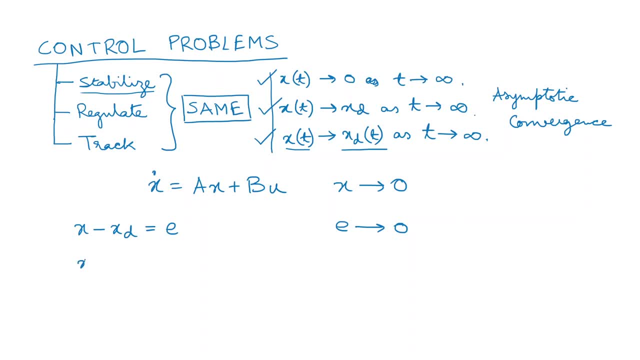 will be to make error go to 0.. In the third case, if you have a state space representation like this, then in the first problem you are trying to make x tend to 0. And in the third case, if you have a state. 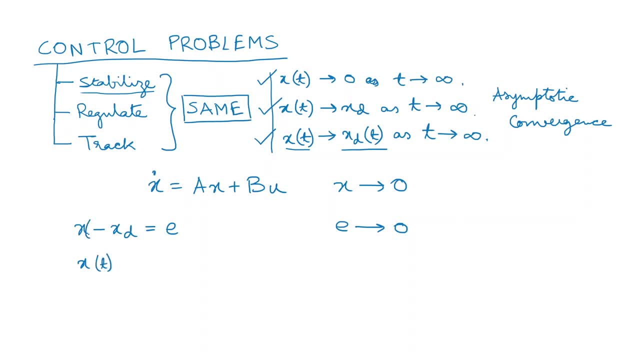 space representation like this, then in the first problem you are trying to make x minus x d and then your intention will be to make error go to 0, right, You can have. this is x t minus x d. this is x t minus x d t. In the third case you can have an error. 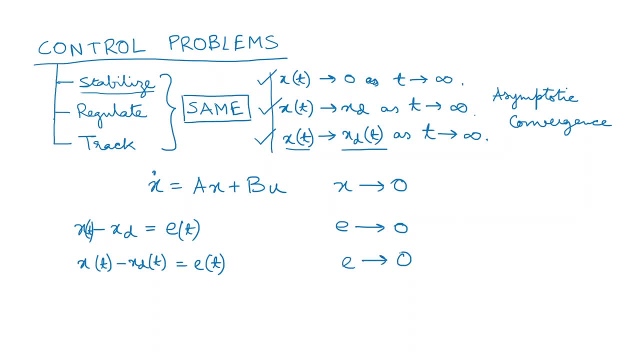 variable defined like this and then your intention again is to make error go to 0.. The first case: you can assume that x d is 0.. If we assume x d is 0, then the first case is also an error going to 0, but the error 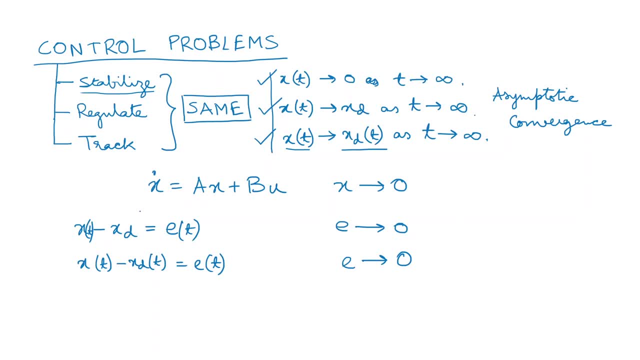 here is the state variable itself. So in all these cases, basically we are trying to stabilize the system. In stabilization, regulation as well as tracking, in all these 3 we are basically trying to stabilize a system. The first case it is the system itself. in 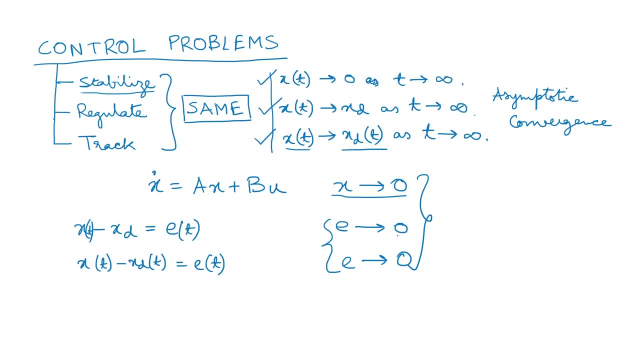 the second and third case it is the. in the first case, it is the. in the second and third case, we are trying to stabilize the error system. So it is as good as to study stabilization only. if we study stabilization, then we are automatically studying regulation and tracking. 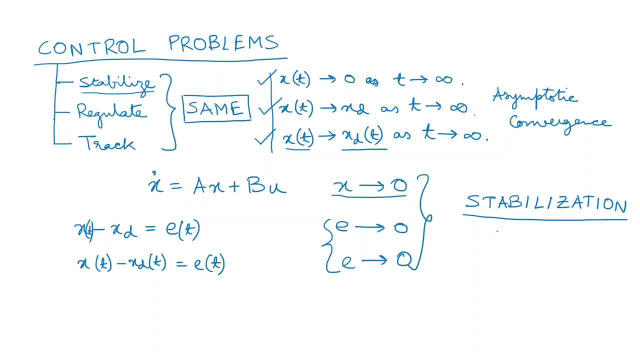 and we would be able to deal with those two problems also. only we have to remember that we need to construct a error variable and go to the error state space. yes, we need to come to the error state space and error state space we need to come to, and then we have. 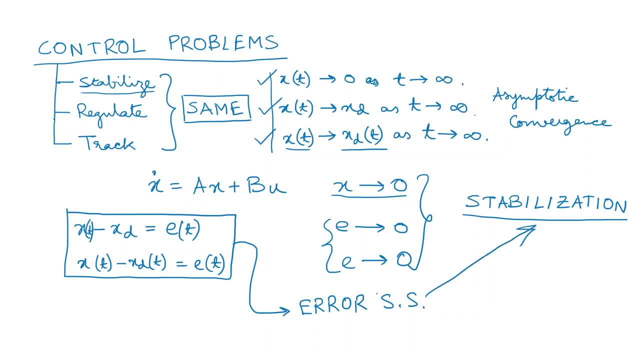 to stabilize the error state space. Let us see the error state space. what? what is the error state space? Is it very unfamiliar to what we are dealing with right now? So for the regulation problem, x t minus x d is the error. what is e dot dot? is x dot minus x d dot? we need to write x. 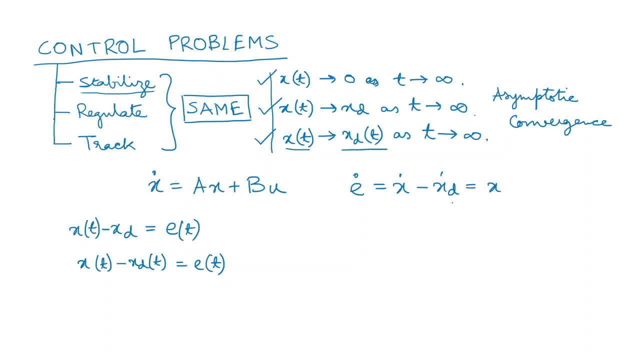 d dot. no, because x, d is constant. it is x dot, E dot is constant. E dot is basically a, x plus b. but what is x? x is e plus x. So I know, we know that this side is e variable, So this side we also should have e variable. So this is basically. 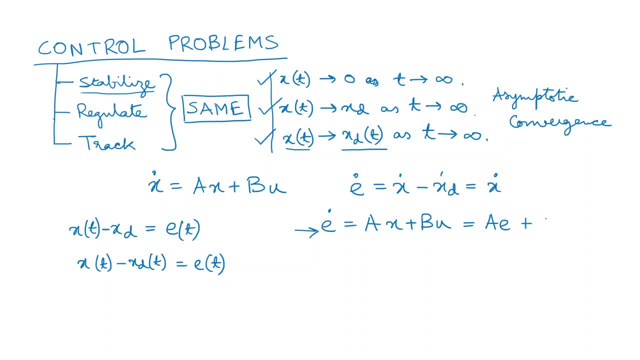 coming out as a? e plus a x d plus right? So this? u? So instead of b? u, you are getting a x d plus b? u now, basically. So in this, in this control action, you can take care of your this, this a x d or I. I can say in this way: 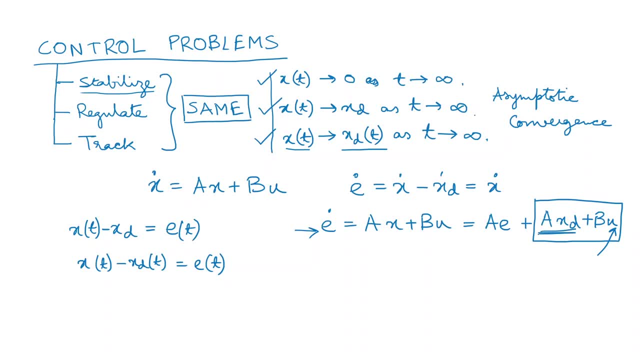 you, since you know this, what is a, x, d? you can always subtract this out from the right hand side by supplying a appropriate control. So, basically, it is in same as your a, e and a, b coming here. so it is same as this particular form, the form of equation. 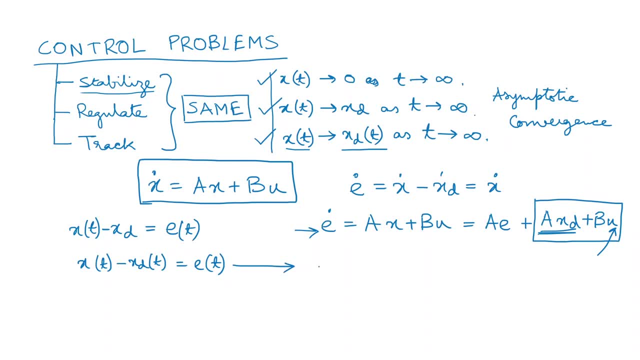 In this case again, if you do e dot, you will have x dot minus x d dot. here you will have x d dot. But that is equal To a x plus b? u minus x d dot. x is what x is: a e plus a x d, a e plus b? u plus a x d minus. 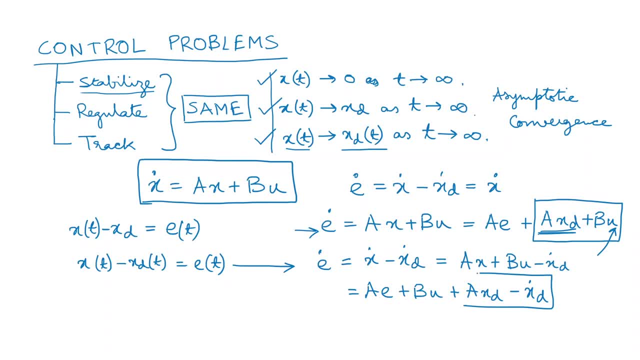 x, d, dot, These two you know. So I should not say subtract. basically you can add actually, So here this thing, so this is, this is what control input you are supplying. I should draw the block diagram. that would explain things better. What is the block diagram here? 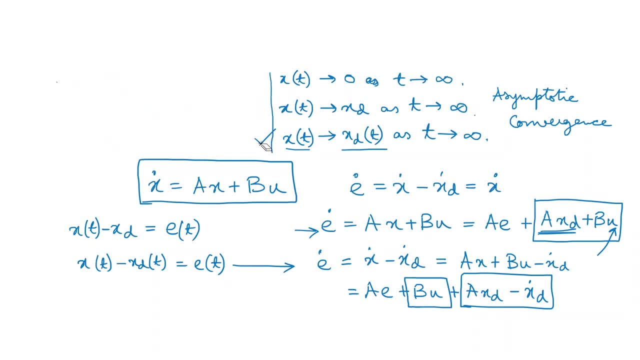 So you have the plant, suppose I am. I am, I am talking about the E plant, suppose I am talking about the error plant. ok, So in the error plant you are having, you are having this integrator 1 by s, whatever is coming out. So this is your E dot From here. 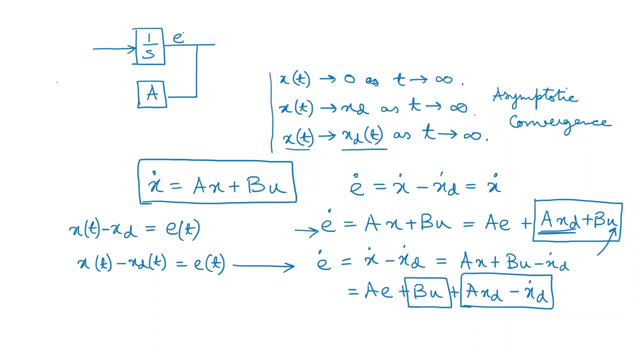 you are taking it as a, your E taking it as a, and then you are coming here. So this is E? dot. What is E? dot? E dot is a, e, a, e plus something which is your b? u right. So your? u, you are. 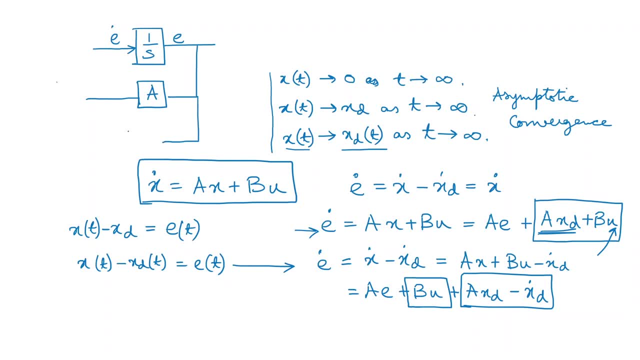 forming using your e, The. suppose there is a controller, So this is our, what we will design controller With this. I am getting a, u and this u. you are passing through a, b right, Adding it to this and you are getting this. This is a normal situation. So if you 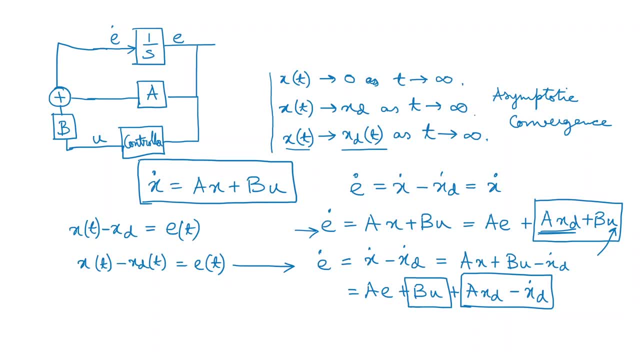 do not have the error. suppose you replace E by x, then this state space equation I have drawn in the block diagram above In case I am getting this error thing, then basically the error system, in the error system I have to add a error. So basically I have to add: 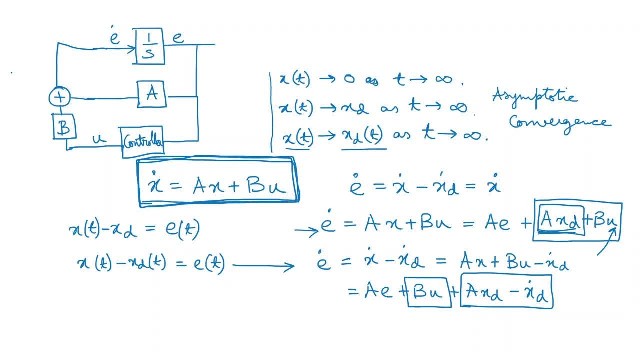 a x d for the regulation problem. So I have to add here, So I can also add a x d here, basically, and then supply, and add a x d here and then supply it to A. Then for the tracking problem, since I know what is my x d t and x d t dot, this I would know because I know. 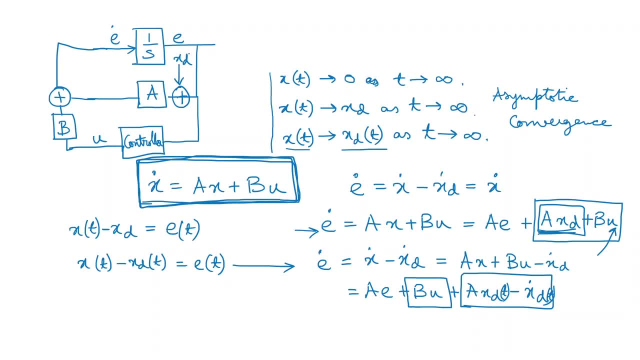 the trajectory. I can supply the x d t here and x d t dot here. That would be my block diagram. So I would… So I would be able to actually provide these additional inputs. These are coming as additional inputs, which I know. I do not have to design these inputs, I already know this. what additionally? 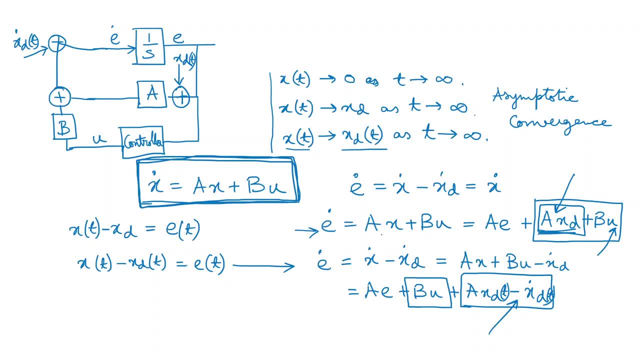 is to be supplied to the error system and I have to design this u only This? u I need to design. So then the problem is basically: I can come back to this problem. I can come back to this problem and solve this particular problem for stabilization. 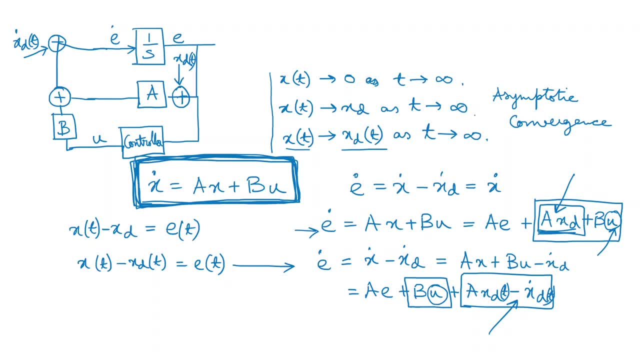 Because these additional inputs which are which I am giving to the systems, these additional inputs which come to the system like this: if I now subtract these inputs from the system, then what remains Is basically this particular system. So the stabilization of the x dot equals to Ax plus Bu system is. 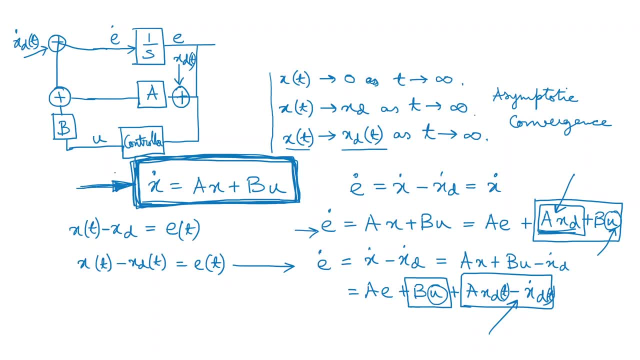 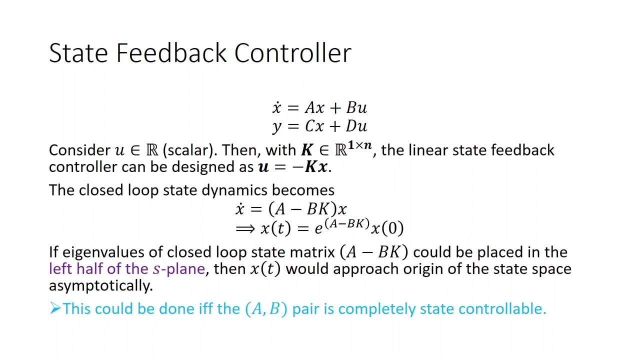 what we are interested to study. That will be sufficient for even regulation and track. So with that idea you would actually go ahead, and here we introduce the basic controller, which is state feedback controller. for our purpose, for our design purpose, to use the state feedback controller. So what is the state feedback controller? 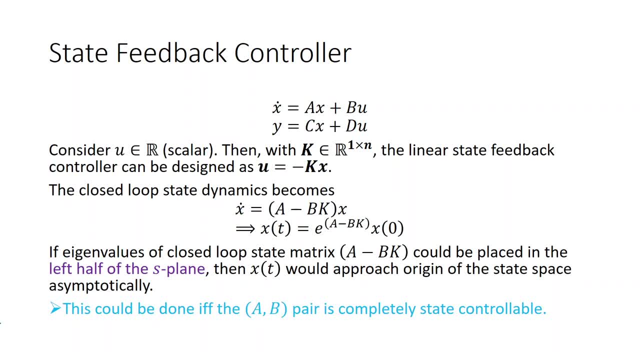 The state feedback controller is basically this. basically this q equals to minus k- Simply a linear relationship with the states. So when you so that is why it is called state feedback. So it needs the information of the states and the states are fed back. So 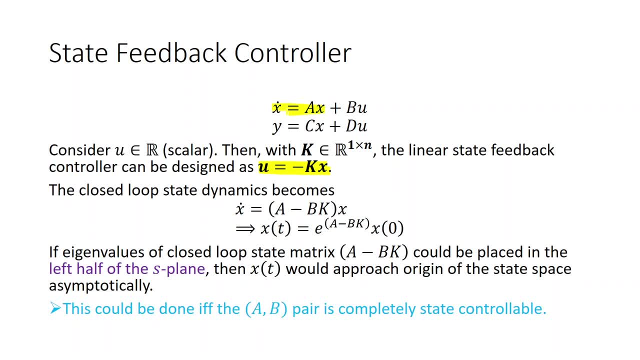 to the system. So originally the system was this: much only. So x dot equals to Ax. this is the same. but you are feeding back the control input with, like this: So you are feeding back, you are taking the states and then then you are. 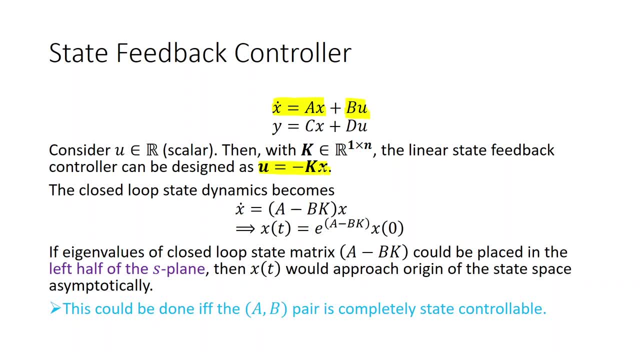 creating the control action as q equals to minus kx, and then we are feeding it back to the system. So that is why it is called state feedback controller. So when you apply this control action, basically what your closed loop system equation will be is. this closed loop system equation becomes this: So it is again. you see it is, it is becoming. 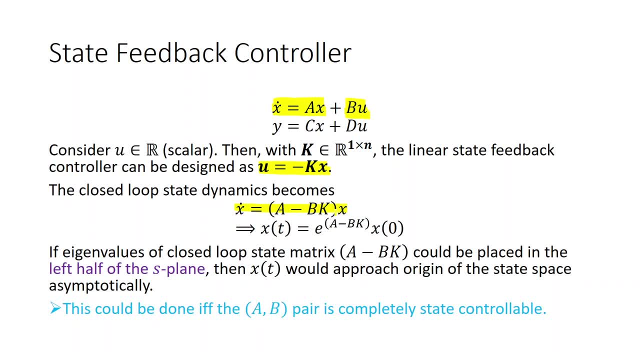 the closed loop system, as if becomes an unforced homogeneous system that we already studied, where the state matrix is no longer a but it is a minus b k. So the solution would be e to the power of a minus b k x 0, and we know that what we need for stability. So 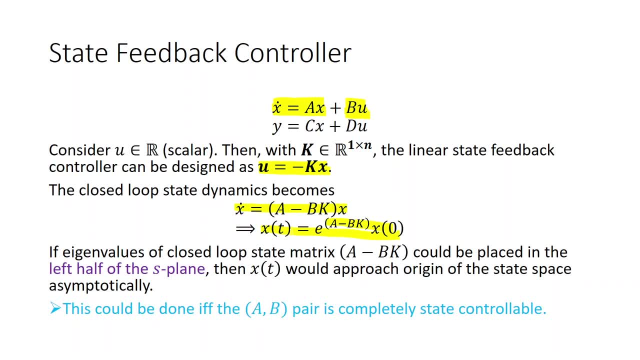 for stability, right x, t tends to 0. we are trying to do that. So for stability, the eigenvalues of the closed loop system matrix in decay needs to be in the left half of the plane. So if you could place them in the left half of the plane using the gain case, this k is in our hand to be designed. 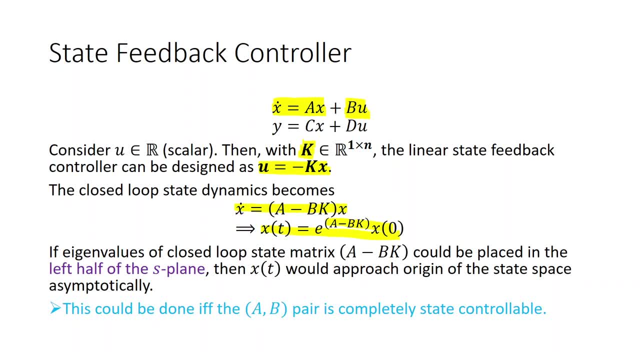 this k is what we need to design. So if we can design a k in such a way that the eigenvalues of the closed loop matrix A minus B k, goes to the left half of the s plane, then our job is done. then x, t will be, will tend to 0 as time phase. So the question is now: are we 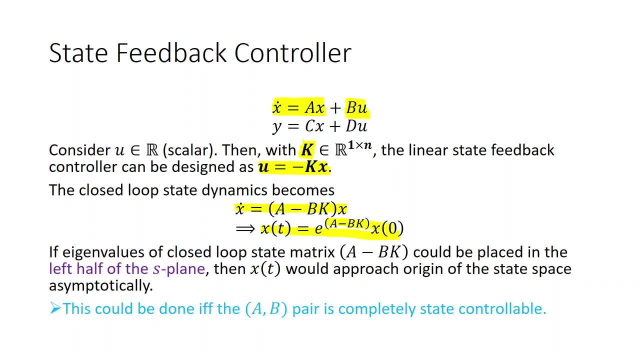 will we be able to design a k like that, That is, taking all my eigenvalues of A minus B k, closed loop matrix, the left half? The answer is that yes, it can be done, but if and only if. a double f if is if and only if. 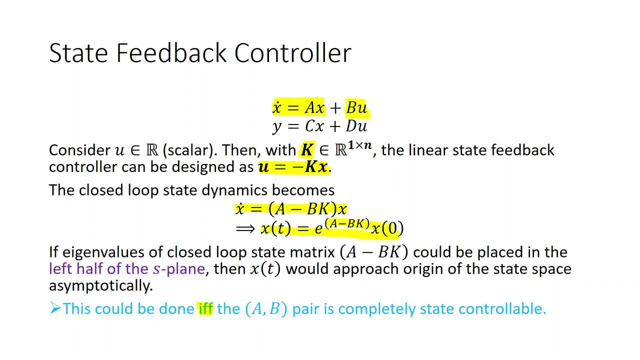 the A- B pair is completely state controlled. This is the condition. that means if A- B is completely state controllable, You can actually design a k matrix which is going to bring us closed loop system eigenvalues. But this statement is not sufficient, because we need to actually know what that k would be. 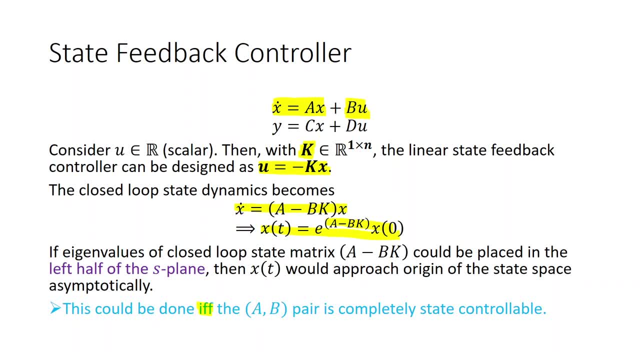 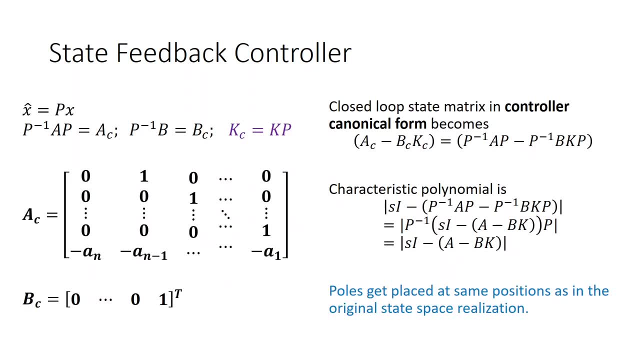 and while knowing what that k would be, we would actually also prove that A- B needs to be state controlled. Let us go ahead into the into looking into the proof. So we would be dealing the system in the controller canonical form. The state feedback controller we will design in the controller canonical form. 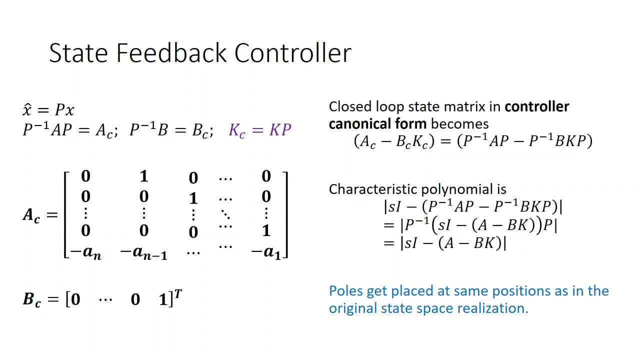 So we would be coming to the controller canonical form using a state transformation, using a transformation, similarity transformation and we would assume that the that we have a gain, we have a state feedback. gain k c equals to k p in the controller canonical. The controller canonical form gain k c is related to the original system gain k. 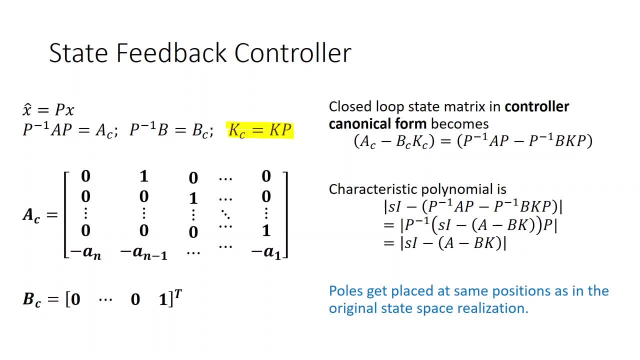 with this relationship, where p is the similarity similarity transfer rate. So if we assume this, then we can see that if I write A c minus B c k c, write a c minus b c k c, which is the. this is the. this is the closed loop matrix of. 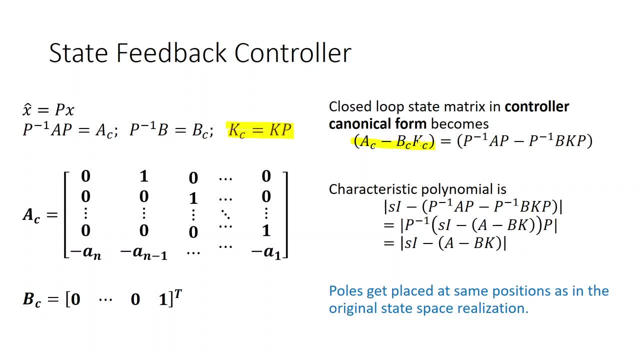 the controller canonical form. when we supply this k, c state feedback control action, Then if you expand, this becomes like this: and then you evaluate the characteristic polynomial of this matrix, of this closed loop system. you see that the characteristic polynomial is same as the characteristic polynomial of the closed loop system, of the actual system. 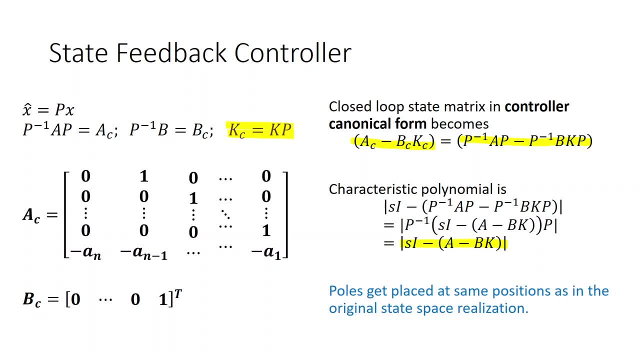 representation which is not necessarily in the controller canonical form. We have started with some representation a b c There. if you apply the gain k, you would get some closed loop, closed loop system representation a b c. So this is the closed loop system which has matrix a minus b k, So it will give rise. 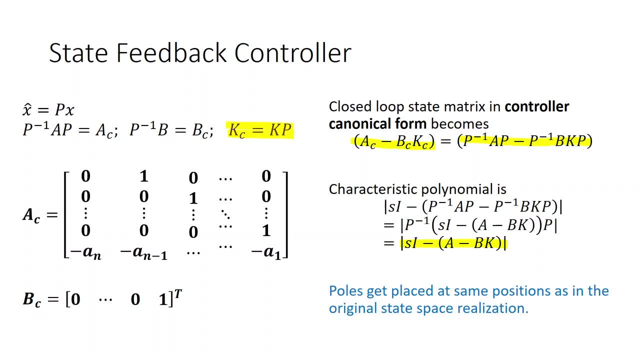 to a characteristic polynomial. Now I see that if I choose k c equals to k p, the controller canonical form, and apply the state feedback gain as minus k, c, x, minus k c, x, x hat here, because we have changed the coordinate x hat, Then the characteristic polynomial of this: 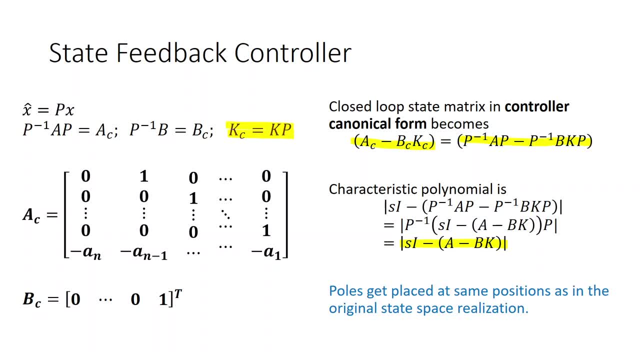 closed loop system will be the same as the actual characteristic polynomial of the actual system. So that means this is a valid. this k c equals to k p is a valid assumption. It does not change the eigen value placement. does not change the eigen value placement. 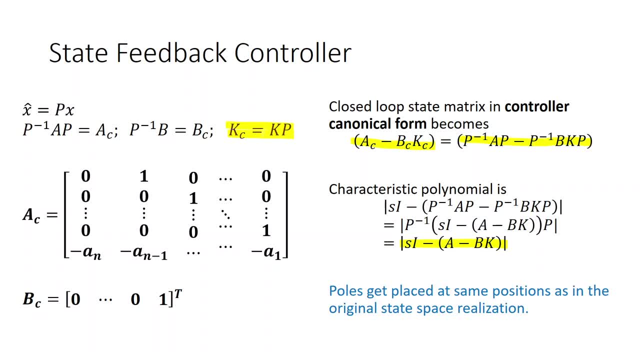 of the closed loop system when we are supplying the control action, controlling action. So this is a valid assumption. So, noting that the controller canonical form is of this form, a, c and b c are in this peculiar manner. This is the peculiarity of the controller. 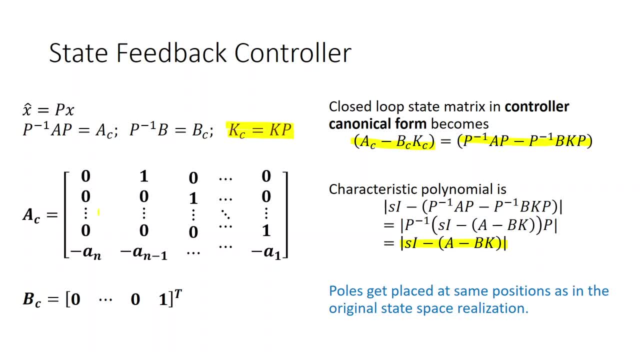 canonical form. This is almost like the phase variable form, right? but b c is here: 0, 0,, dot, dot, dot. So noting that the controller canonical form is like this. So here, the controller canonical form is like this. So let us see what happens when we supply the 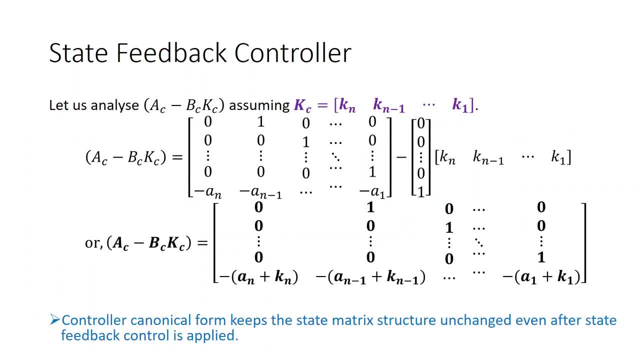 state feedback controller k c. Suppose I take my k c as like this: This is the vector. k c is a vector, assuming that my control input is a scalar control input. We are trying to make a scalar control input, So this k c is like this. So when I supply this k c, 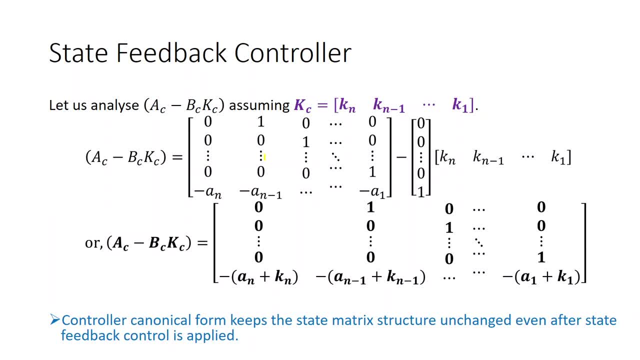 then a, c minus b, c, k, c becomes like this and you see only what happened. basically This: a, n, a, n minus 1, these coefficients in the last row of the a matrix, they simply get changed by including the k, n, k, n minus 1, these gains, They simply include or append the gain. 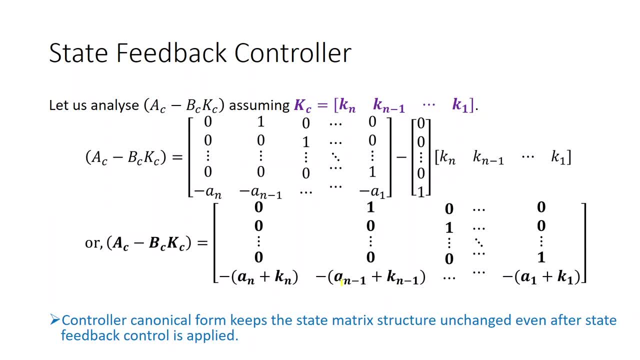 a i's into themselves and nothing else changes. So the controller canonical form keeps the same matrix, state matrix structure unchanged, even after state feedback controller is applied. That is the peculiarity of the controller canonical form. Controller canonical form is such a form where, even after state feedback, controller is applied. 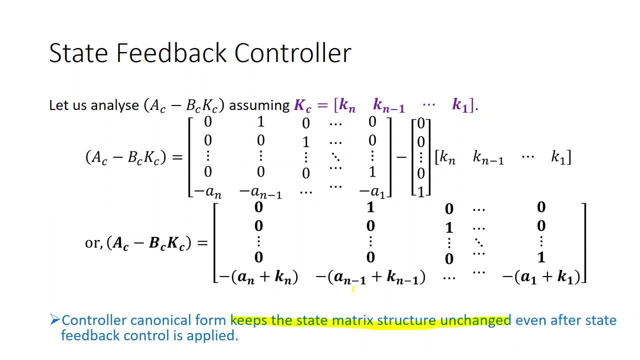 the state matrix structure remains unchanged. State matrix structure form remains unchanged. That is the controller canonical form. What happens? what is the utility of this? The utility is very straightforward. If I ask the question: what is the closed loop characteristic polynomial, Can you tell me? You will say yes, it is very obvious now, because I know that the state matrix 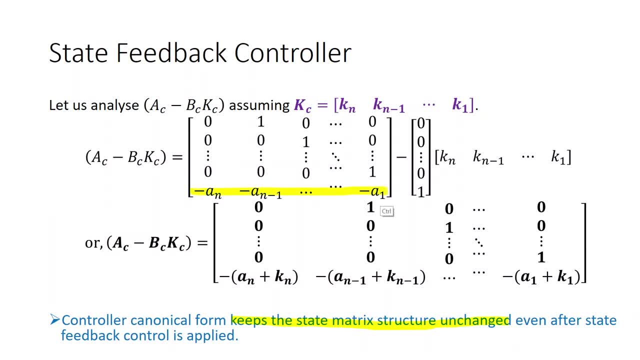 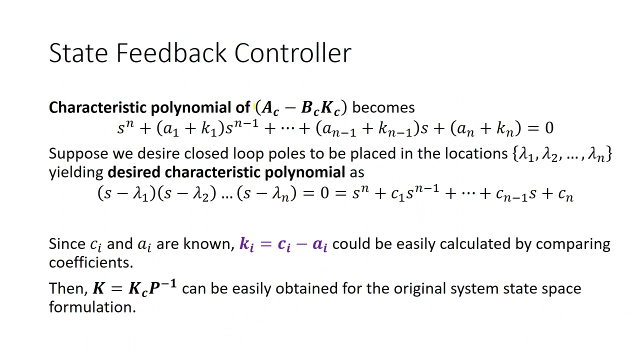 that the correct. the coefficient of the characteristic polynomials are these: last row elements: the controller, canonical form, So the, since the form does not change, the closed loop coefficients, closed loop characteristic polynomial coefficients are these: So the characteristic polynomial of the closed loop, AC. closed loop state matrix, AC. minus. 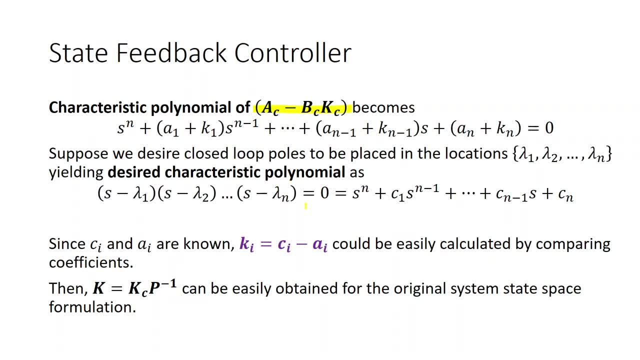 LBCKC. they are these, and if we desire the eigenvalues to be placed at some particular location, then we can actually form a desired characteristic polynomial always. So this lambda 1 to lambda n, let them be the desired location of the eigenvalues. then I can always. 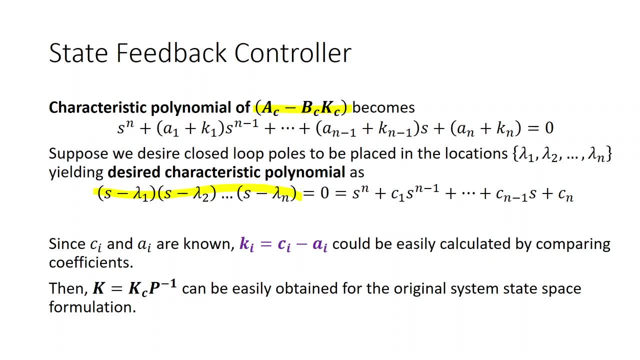 have the desired polynomial. So if I get desired characteristic polynomial, I simply need to extend this and I will get the desired characteristic polynomial. Suppose they are: the coefficients are c 1 to c n, then if I wish that with my gain, Kc applied the controller canonical form, I would get the. 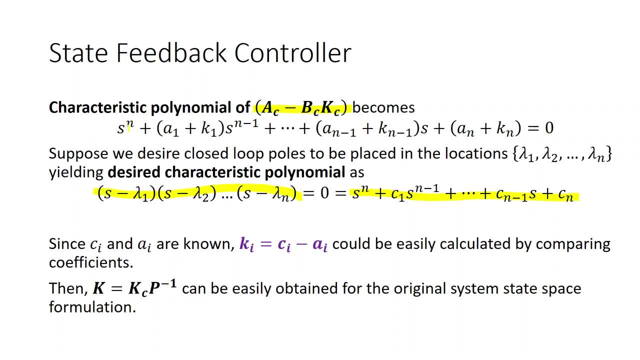 desired characteristic poly � ,en same as. . the closed loop characteristic polynomial closed loop characteristic polynomial same as the desired characteristic polynomial then what do i need to do i simply need to match the coefficients i simply need to match a1 plus k1 with c1 a2 plus k2 with c2 etc etc 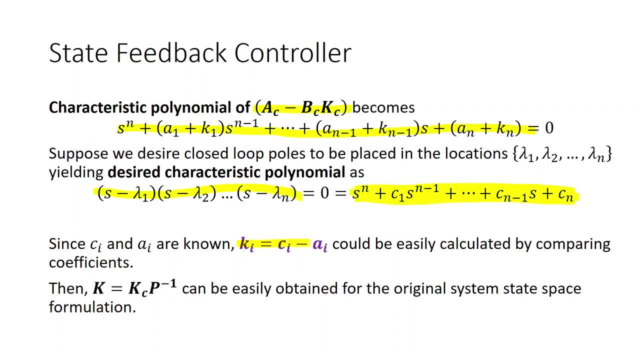 and in that matching i can get what my k i for all the i's: a1 would be c1 minus a1. k2 would be c2 minus a2, likewise. so now when i have got all my k? i's, i can now calculate back the state feedback control. 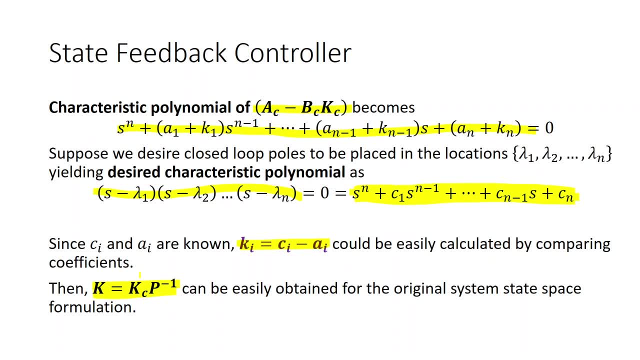 again k of the original state space representation. so So nice, so easy, right so easy. but one thing we have not done: what is this similarity transfer? This we need to know, otherwise we will not be able to do the calculation. 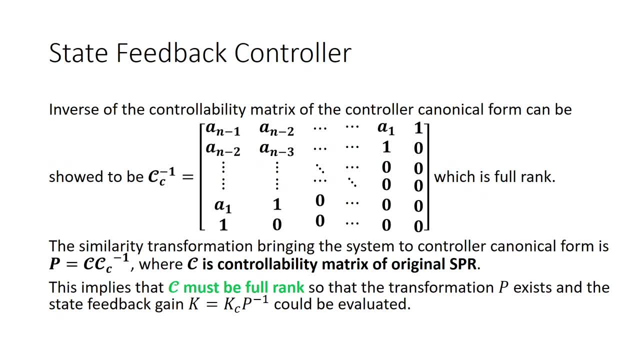 Let us put this as a fact. you can take it for third order system or fourth order system. probably you will be able to do it. you can check it that the inverse of the controllability matrix of the controller. canonical form inverse of the controllability matrix of the controller. 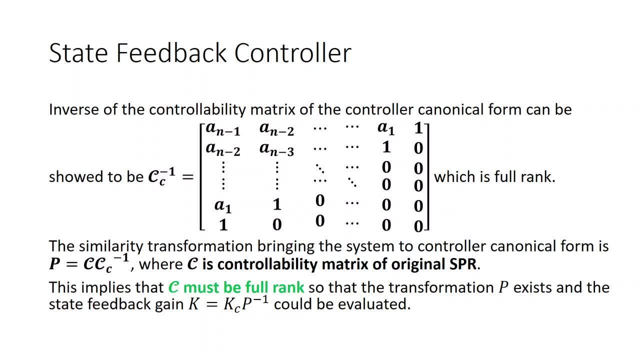 canonical form would be, of this form would be this: So this is the form of the inverse of the controller: controllability matrix of the controller, canonical form and of course this is full rank. of course this will be full rank, as you can see from the structure and hence the, you can always calculate the similarity transformation. 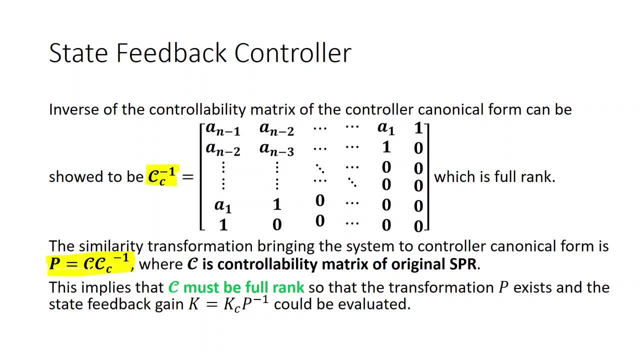 P. know the controllability matrix of the original system, you can calculate the similarity transformation P. Now, also to note that, since you are talking about a similarity transformation, that has to be non-singular, and your inverse of the controllability matrix of the controllable. 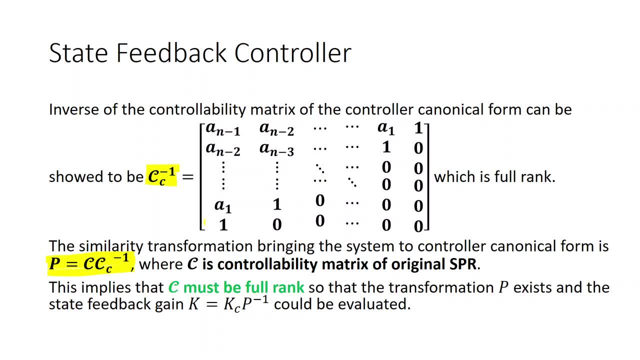 canonical form obviously is non-singular. your controllability matrix of the original state space representation must also be non-singular. that means of full range, must be of full range. This means the original state space representation must be controllable. the A- B pair there must 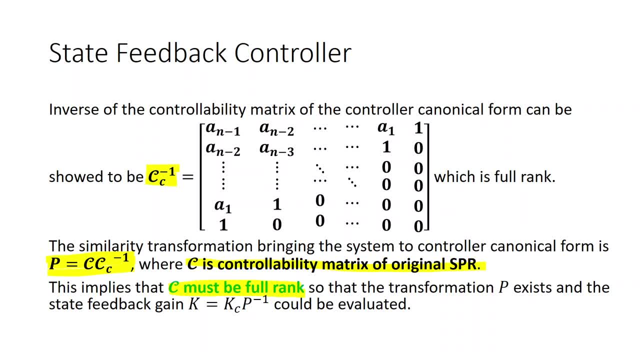 be controllable. That is how we prove the controllability matrix, Controllability also, that controllability is required. you also come to understand how we can actually find out the gain of gain of the gain K of the control action state. 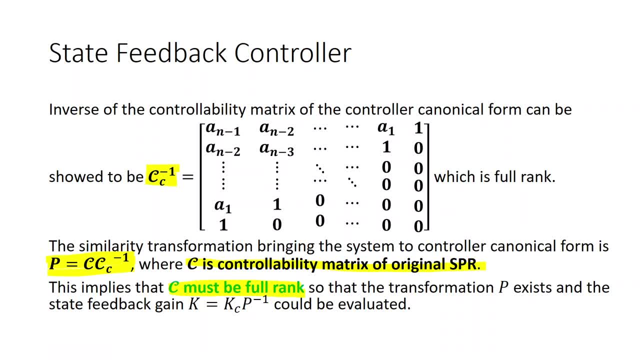 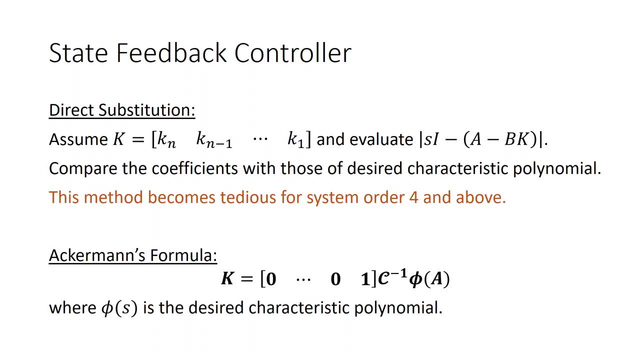 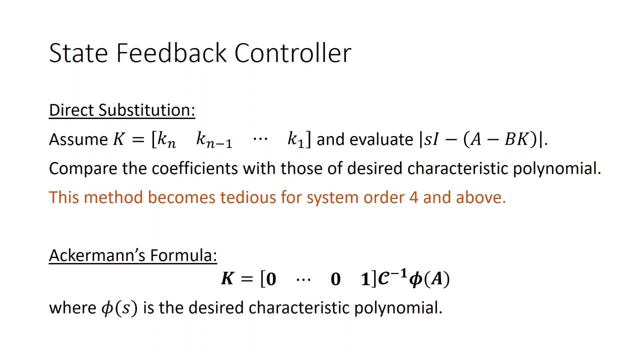 I can especially say that this method available well, this method available well, that wise it you can also take away. it is accessible to a group of type expression. Then chicken out, chicken, ada, Yeah. Now what is the new method of looking for the conformal space distribution? 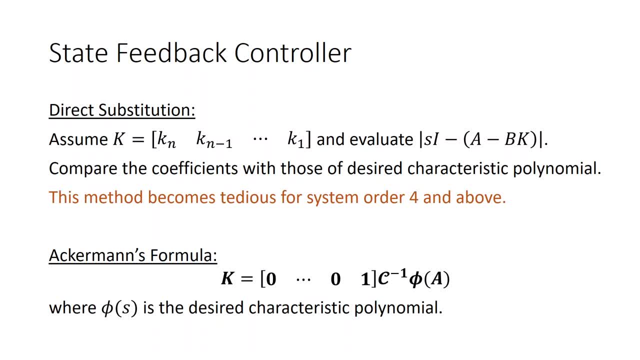 How you looking. do that? Does that way you can nutzen our methods during calculation, Using neither of these methods. Now, starting from theests The second, The first go to the controller. canonical form, actually So straight away: d? d for any state space. 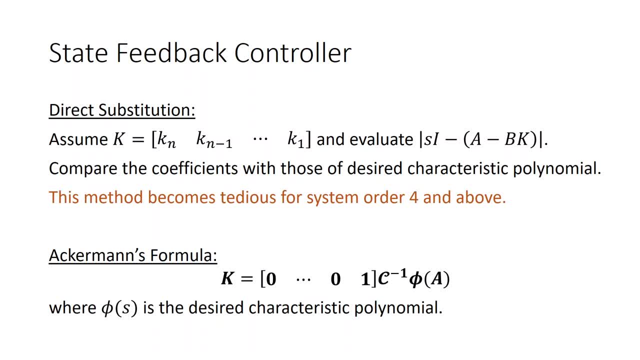 representation d, d. However, this method becomes tedious for system order 4 and above. So you have to calculate the characteristic polynomial of this a minus b k matrix, which is not very straightforward. In controller canonical form it is straightforward, but otherwise it is. 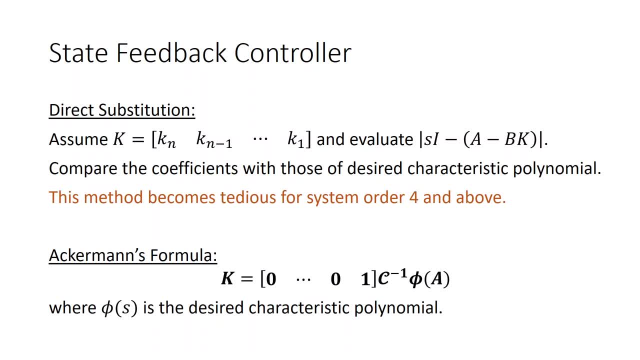 not straightforward. So you have to do the calculation, So it becomes tedious. for system order 4 and above, The other is Ackermann's formula. So here you can simply remember this formula. There is a derivation which is long, So I will not go through that. So 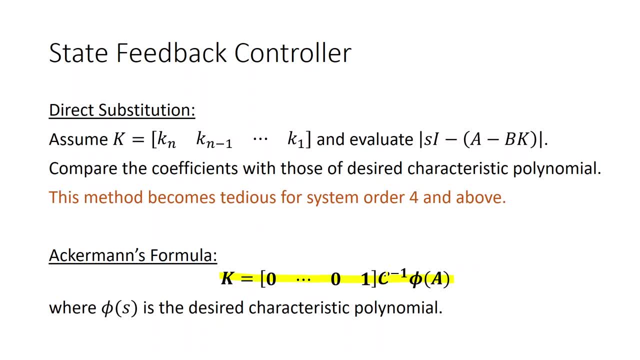 simply remember this formula: This is 0, 0, 0, 0, 1.. So this is the length of n, n being the system order. So all n minus. So all n minus 1, 0s, and then a 1.. Then what is C inverse? C is the controllability matrix. 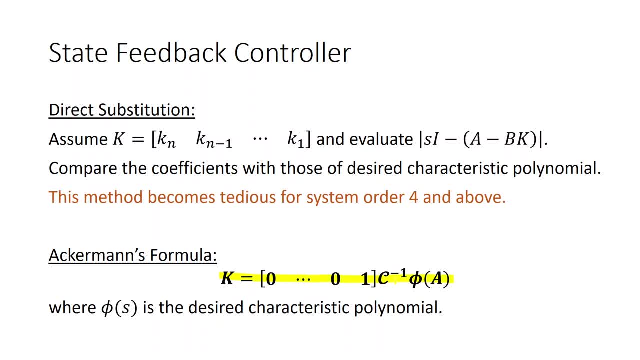 of the given representation. inverse of that, What is phi A, Phi S is the desired characteristic polynomial. So always have to go to the desired characteristic polynomial. You have to find that. in any case, in any of these methods, you have to always find that. Is that you know? 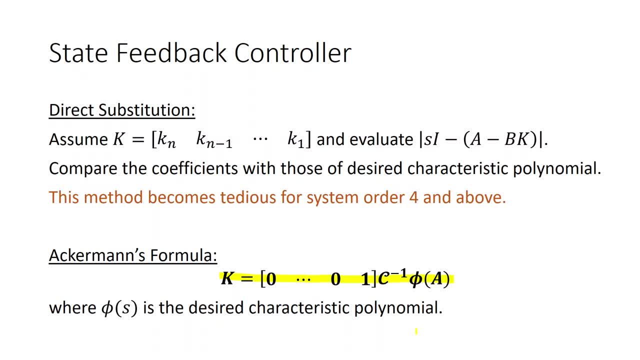 You know where you want to place the poles, The exact location of the poles you can actually give. So you will obviously give some locations in left half plane, So some location. whatever you choose, or whatever is given by the given in the problem to you, you can find out the desired characteristic polynomial also. So 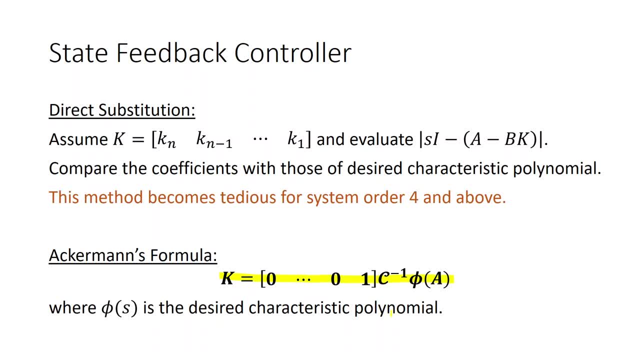 you find out the desired characteristic polynomial. but in place of S, to replace with A, which is the state which is the state matrix of the pole. So you can find out the desired characteristics of the original system. the open loop state matrix, You replace phi. 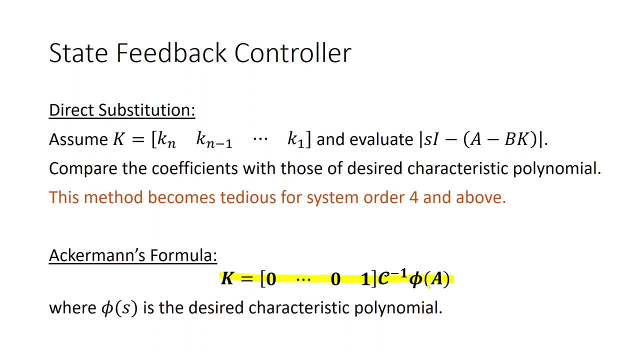